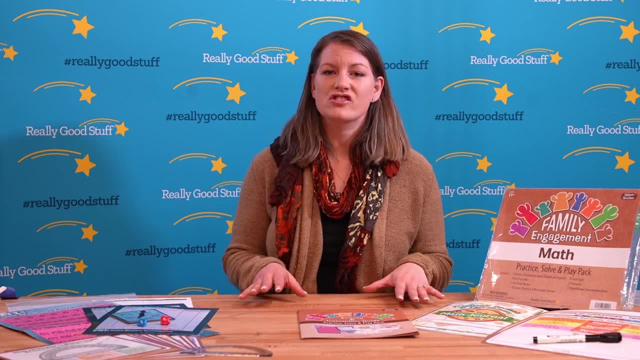 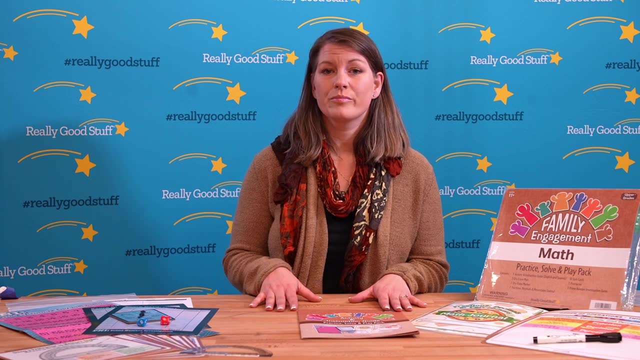 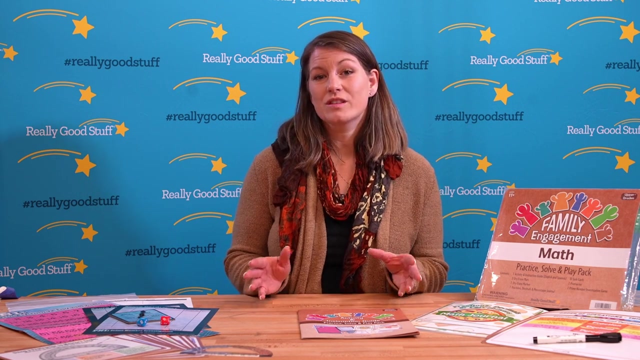 summer camps. It could even be extra resources for teachers in a classroom or hands-on materials for digital learners at home, But this kit would be great for students to take home and engage with their families, and it has all the materials they need to connect with the families and to build. 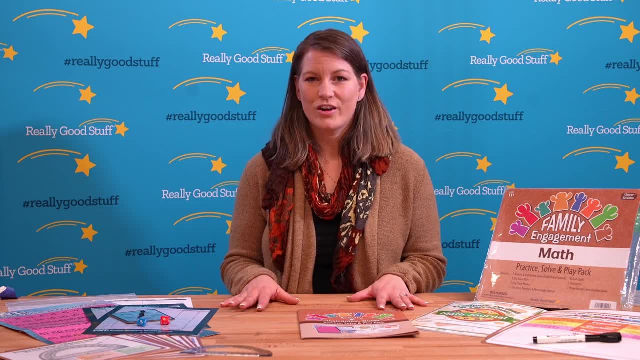 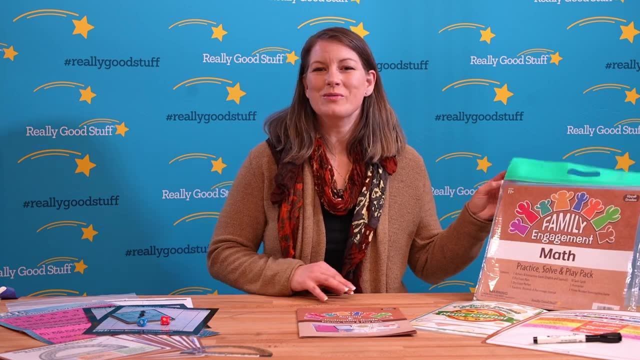 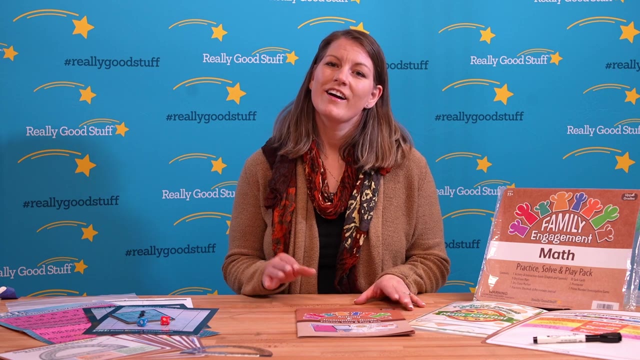 that school-to-home connection that we're all looking for. The kit comes in a sturdy handle carrying bag so when students go from school to home they can keep all their math materials in one place and keep them safe and dry. The cornerstone of this kit is this activity, and 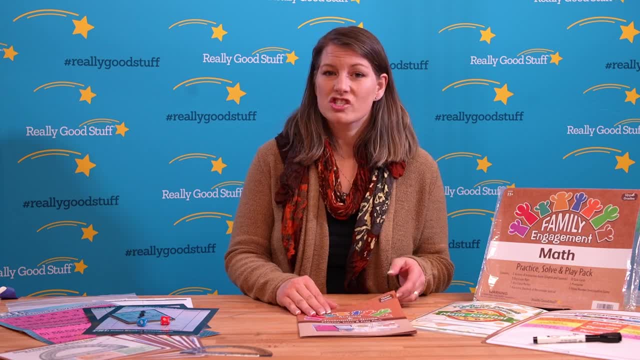 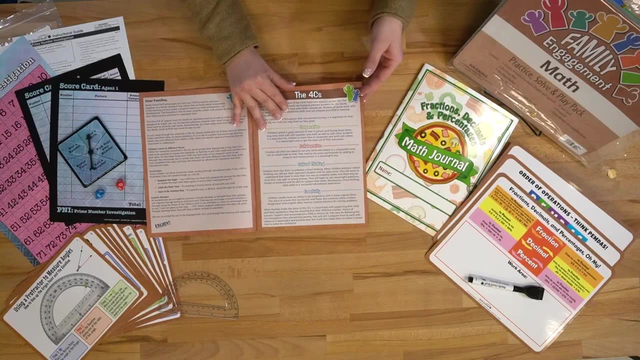 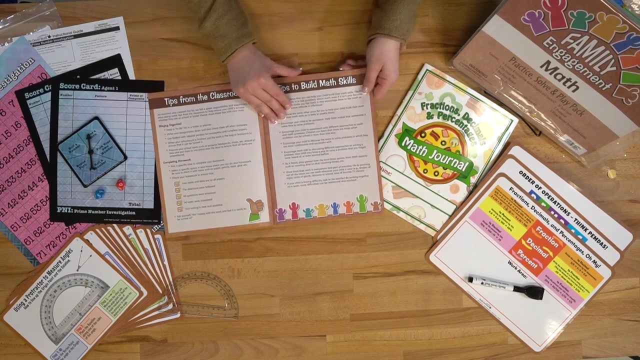 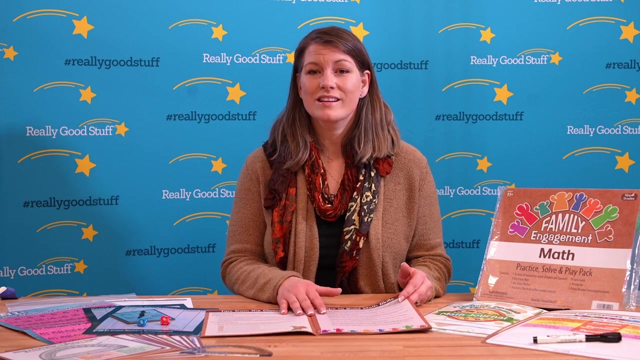 instruction guide. This 24-page color guide is written equally in English and Spanish. It features a parent letter or a family letter, the four C's tips from the classroom and tips to build math skills, And we find that when we send this type of information home to parents and they 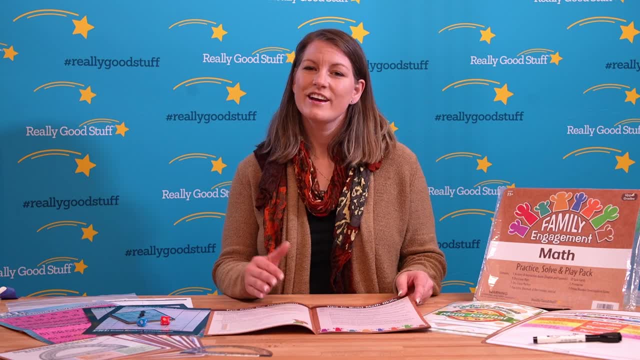 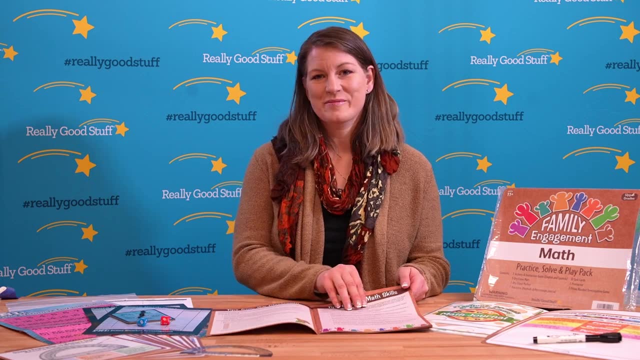 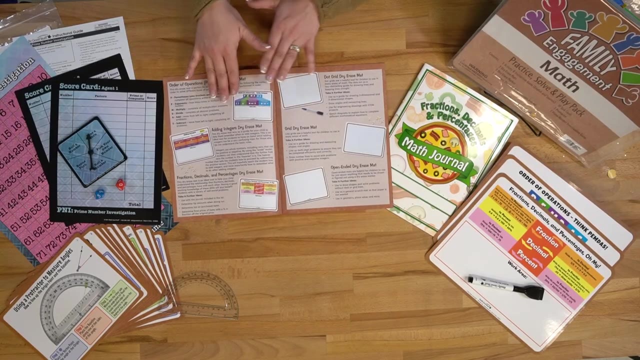 feel like they know how to best support their child. it really gets them involved and helps get the child excited about math and set up for success. This guide will also walk a teacher or the parent through how to use each item in the kit. So here on this page. 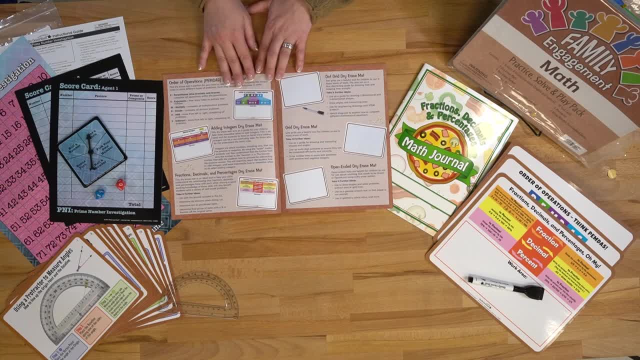 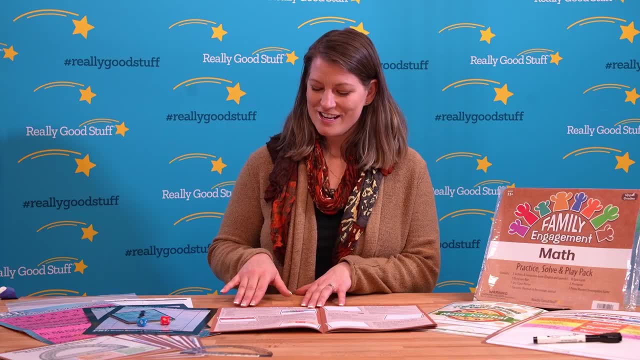 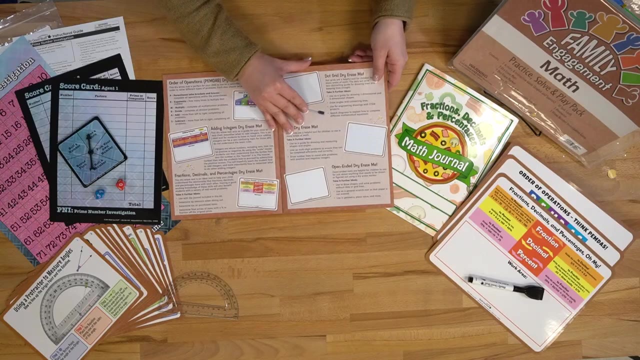 you'll see it's walking you through our three double-sided dry erase mats for choice. the fun. This grade for the upper grades features the order of operations mat, the adding integers, mat, fractions, decimals and percentages, a dot grid, aligned grid and an open-ended grid. 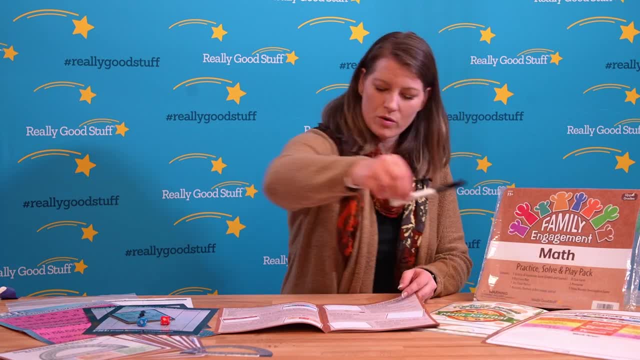 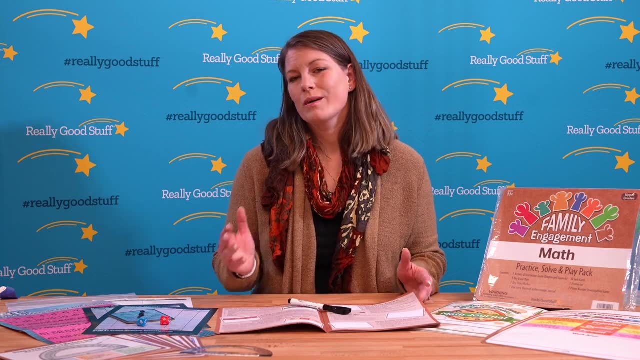 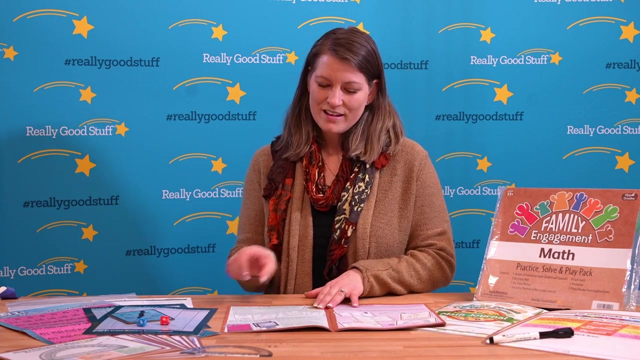 Now these boards will also come with a dry erase marker, because we know that not every family is going to already have one at home. We want to set the kids up for success and give them everything they need, so that marker is provided right in the kit. This kit also features a fractions decimals. 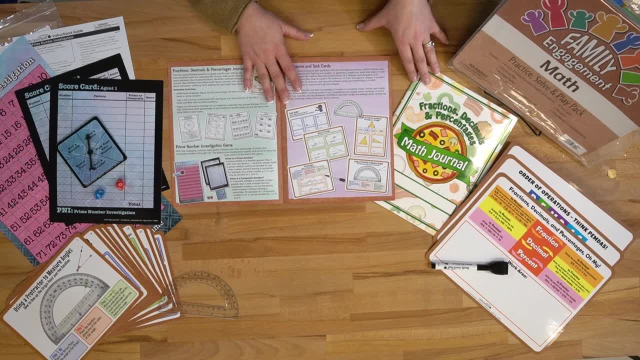 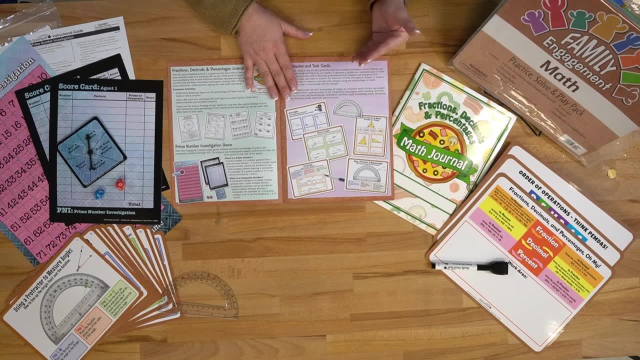 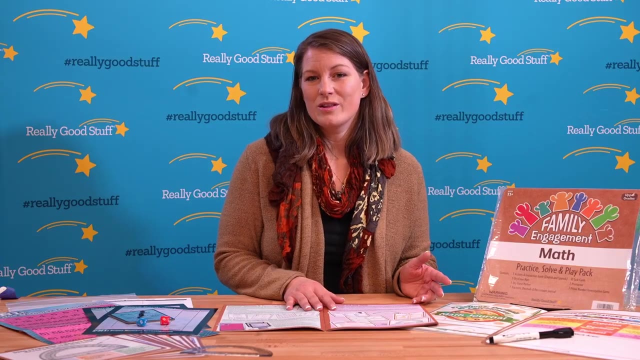 and percentages journal. And what's fun about this journal is it has a pizza theme and it tries to show that fractions, decimals and percentages are in every business. They're in buying and selling and it's all around you when you're out in the world. So that real life application is where 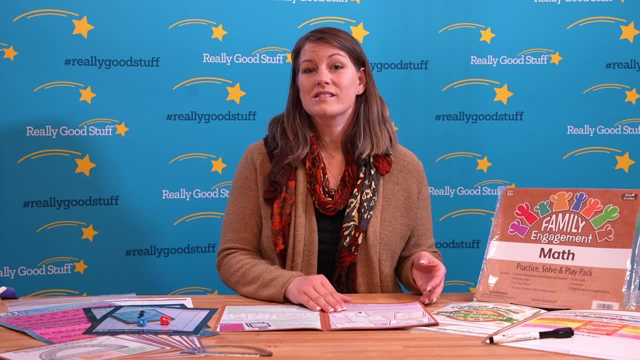 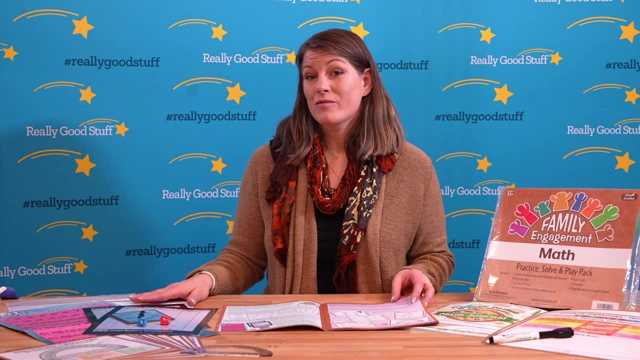 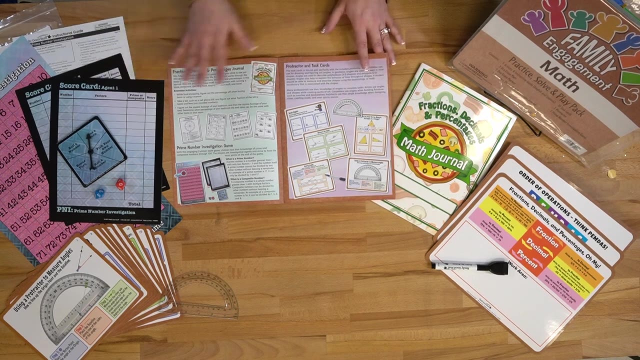 students start to buy in and see the purpose of learning and really get them invested in their own learning. The kit will also include this game for two players: the prime number investigation, where students can look at the difference between prime numbers and composite numbers and the difference between the two numbers and the difference between the. 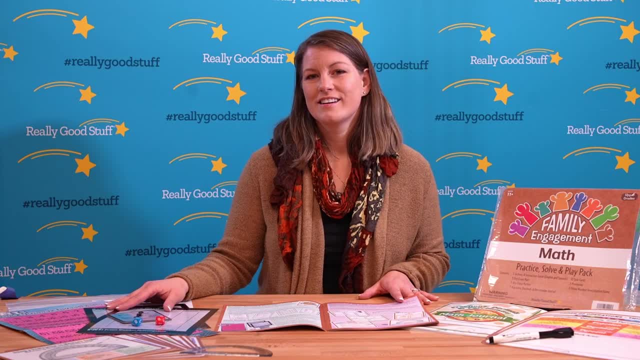 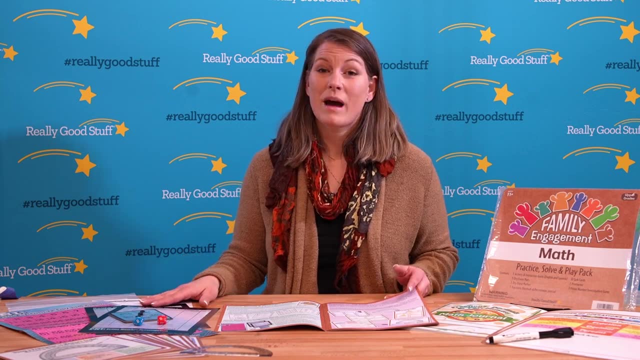 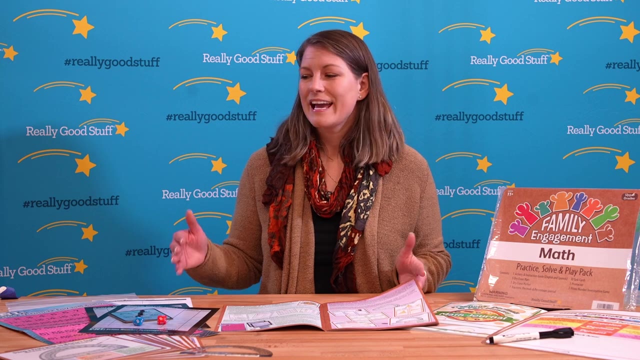 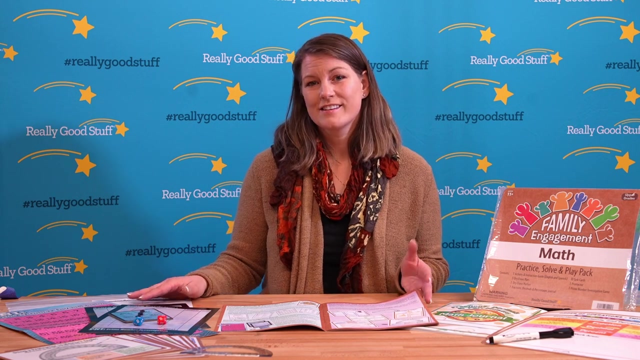 prime numbers and composite numbers. So it's a really fun game to play and I hope you have a great day. Thank you for watching And I hope you have a great day, Bye, bye. So we love to include social emotional in our curriculum whenever possible. 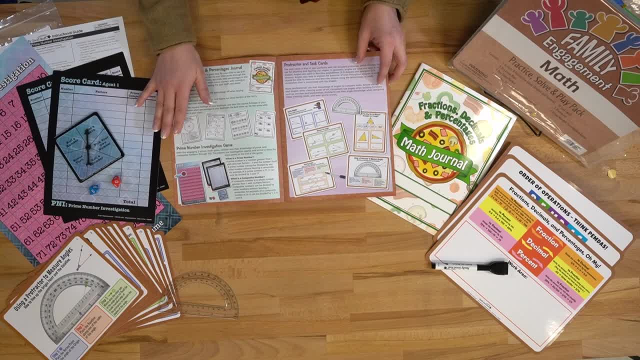 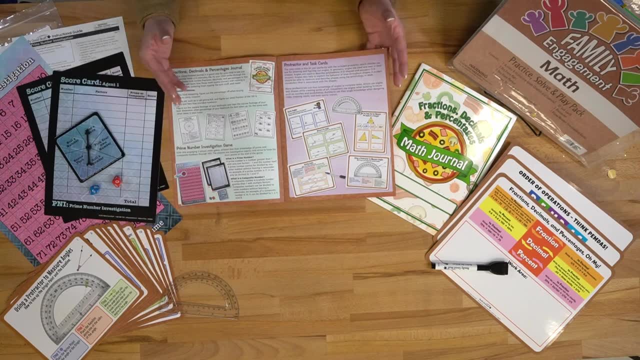 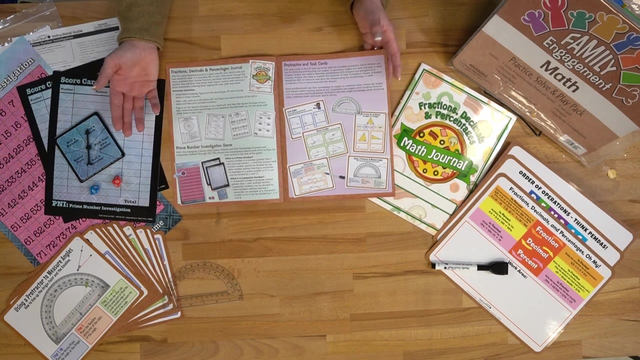 The kit also includes 10 double-sided task cards, and these task cards focus on angles and how students are going to see angles throughout their life. They learn to measure angles, to find angles and even find the area of certain shapes using that protractor. The cards are laminated so students 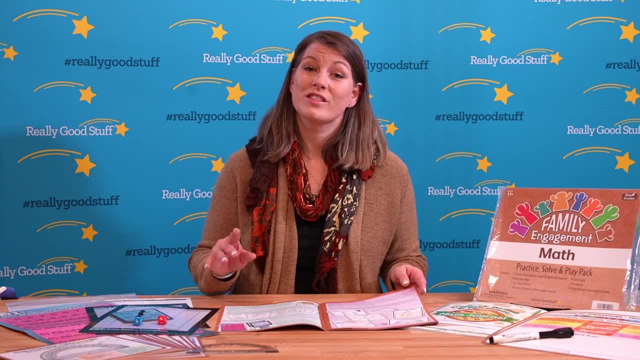 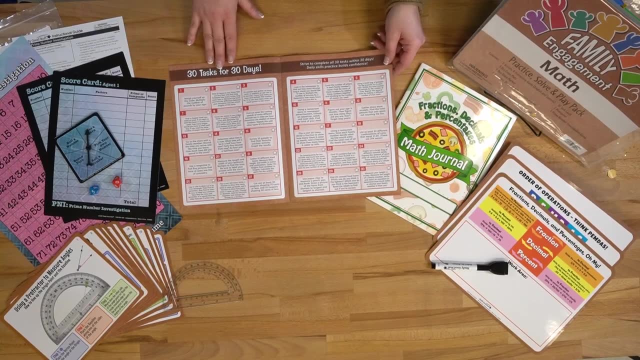 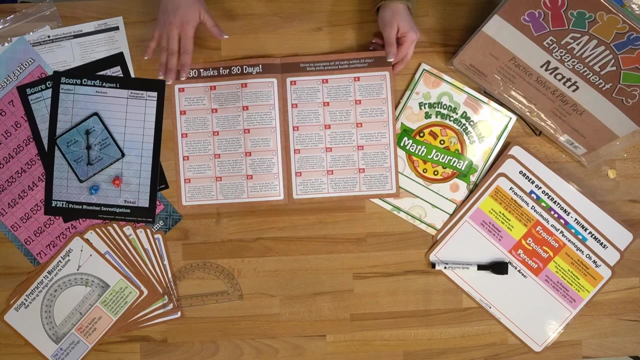 can even go beyond using the protractor and write down their answers with the dry erase marker. The guide also features a set of learning goals and a 30-day calendar. This calendar of activities is fantastic for a family to do one per day. It won't take them a ton of time, but it'll get them. 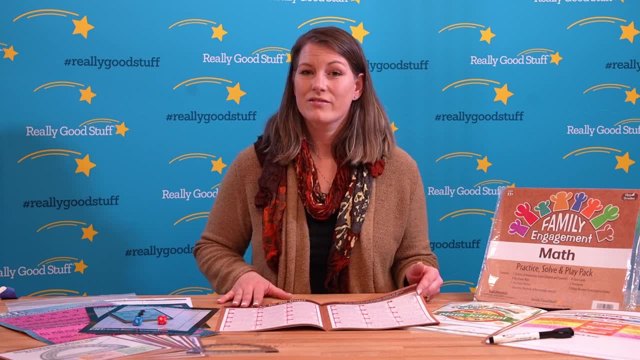 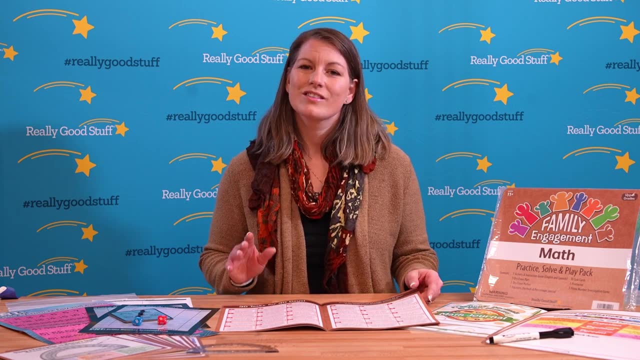 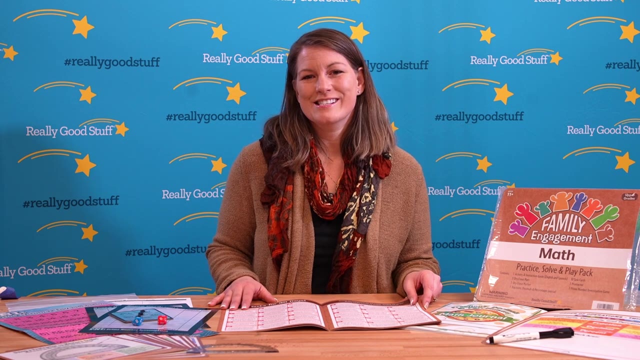 connected and talking and including math in their life. When students engage in these math concepts every day and start practicing daily, they'll start building that math fluency and confidence that we're all going to have. So let's set our students up for success and provide them these family engagement kits.